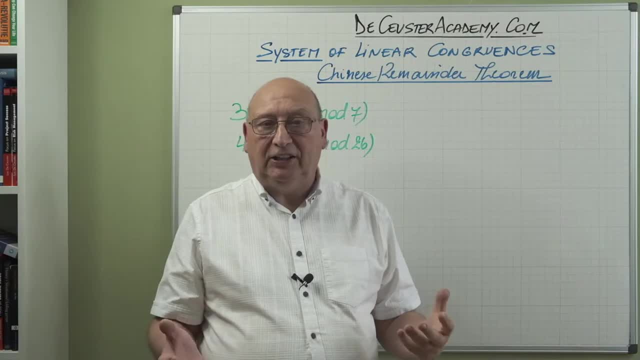 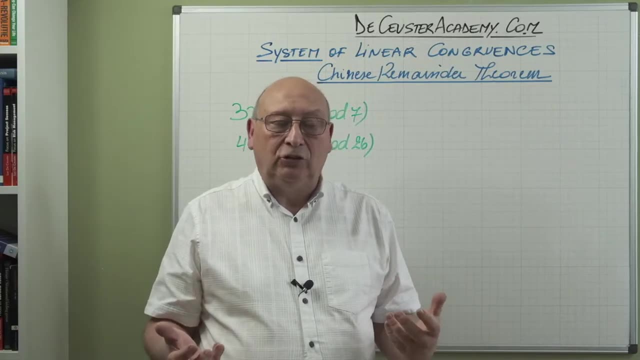 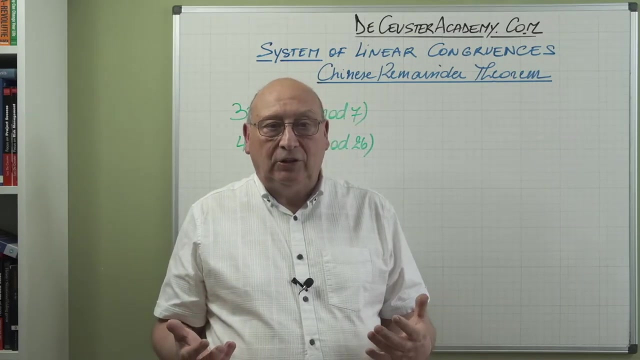 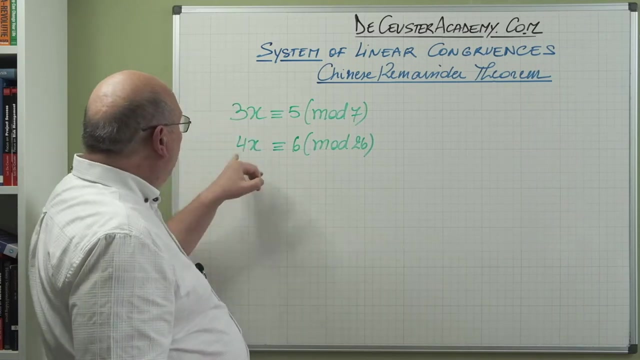 the previous videos we looked at the classical approach to the Chinese remainder theorem and we had linear congruences of the form. x is congruent bi modulus mi and the x coefficient, or the coefficient of x, was equal to 1.. In this exercise we have it a little bit different. We have 3x is: 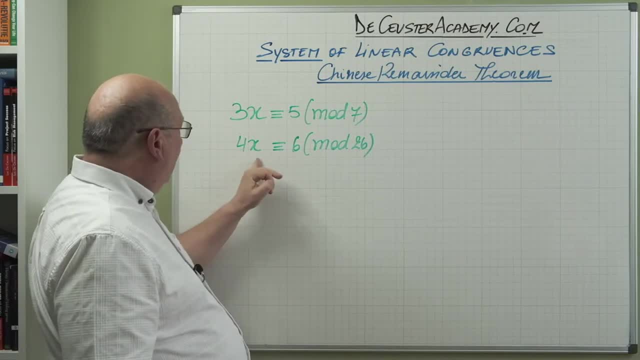 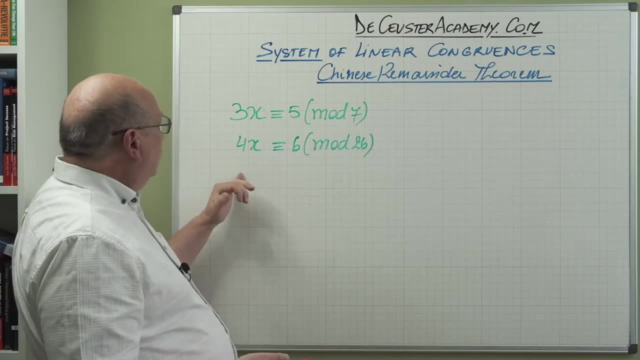 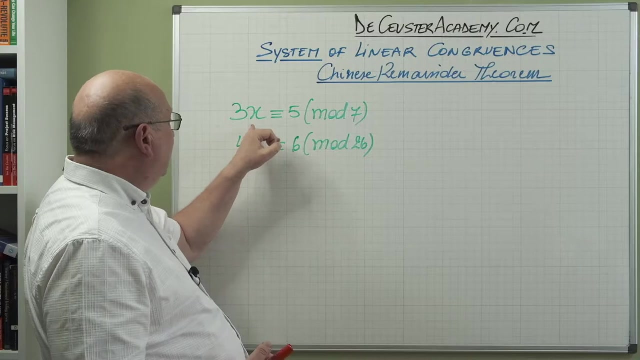 congruent 5, modulus 7, and 4x is congruent with 6, modulus 26.. The first thing that we have to do is, in fact, transform these equations in the form, in the classical form. So we have to transform. this is: x is congruent with a. 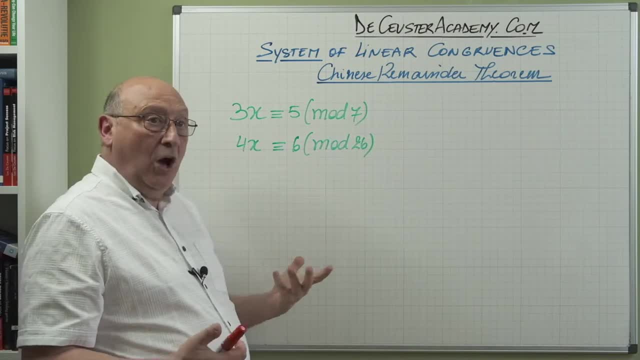 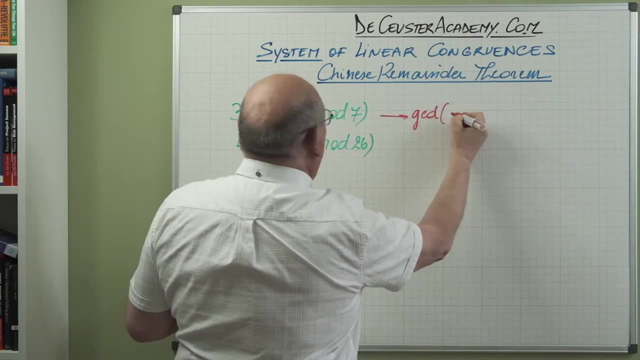 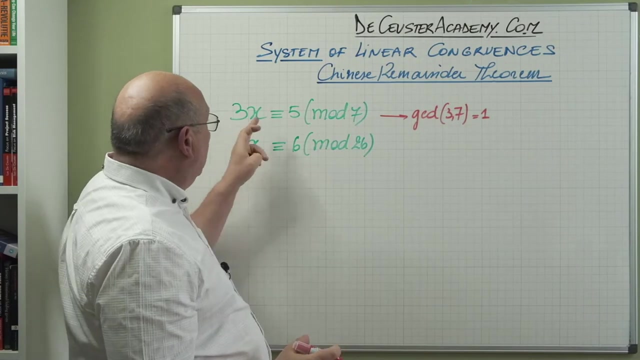 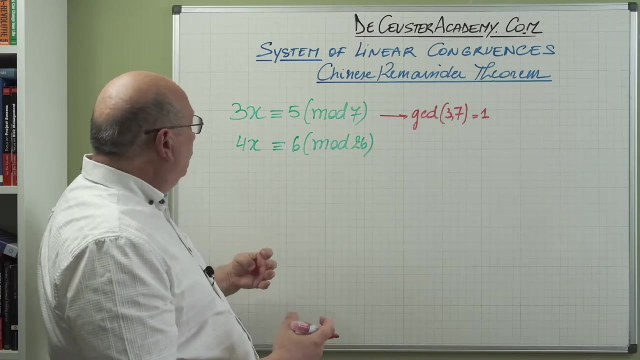 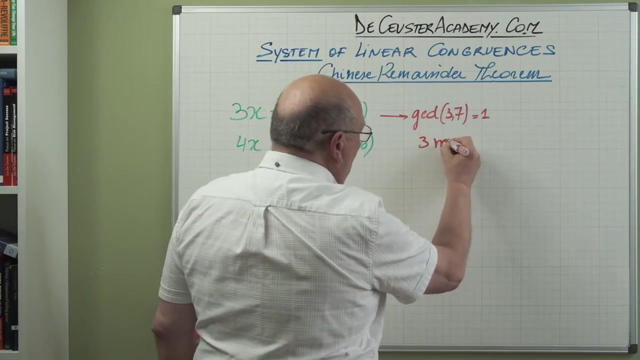 constant modulus 7.. Now, when we look at this, what we see here is that the GCD of 3 and 7 is equal to 1, which means that the 3 modulus 7 is inversible, And what we can do now is to find the modular inverse of 3 modulus 7.. So we have 3 modulus 7. 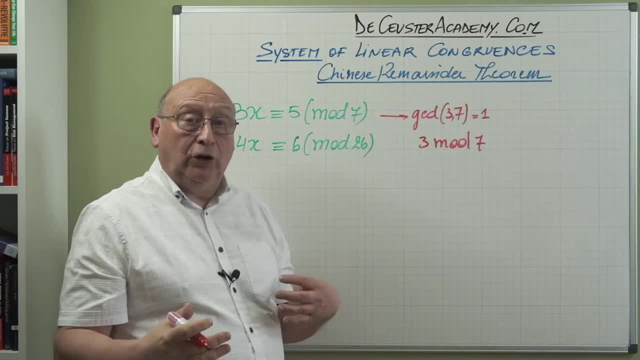 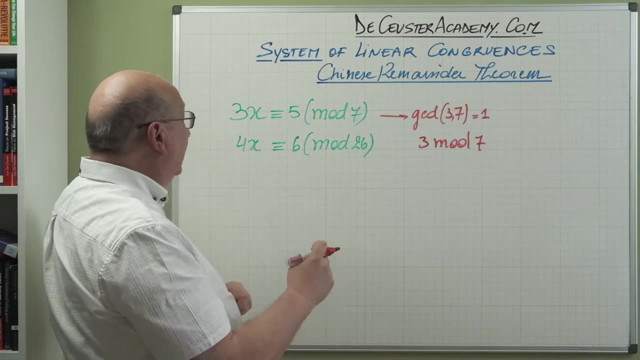 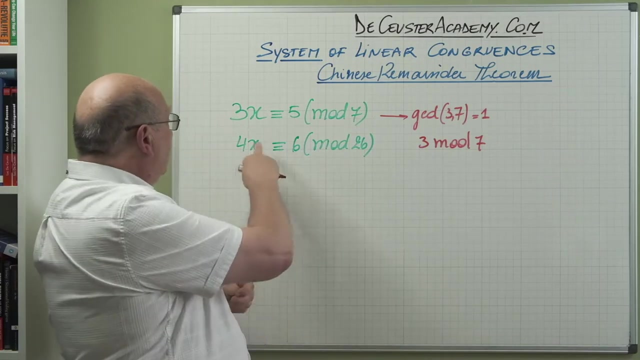 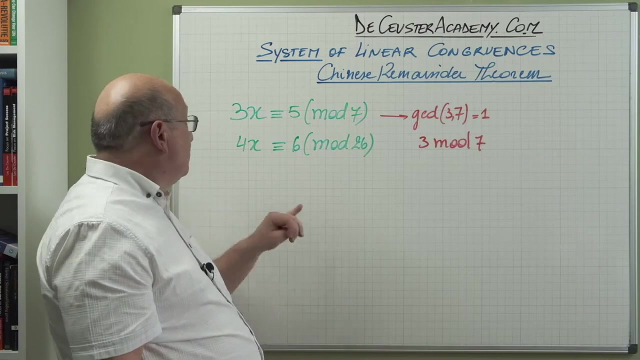 and we have to find basically the modular inverse. Now when we look at this, we can already see what we have here, and when you get a little bit more experience in these calculations you can immediately see. when I multiply 3 with 5. 3 times 5 is 15 and 15 modulus 7 is equal to 1.. So when we say 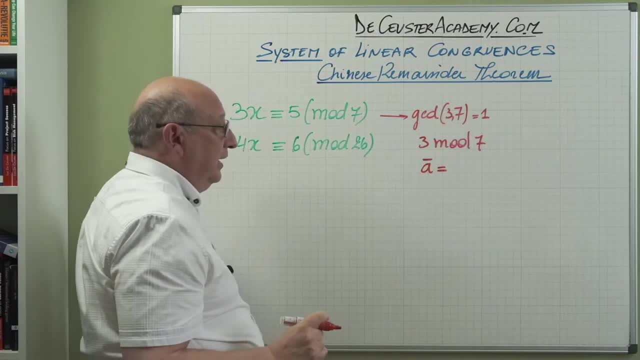 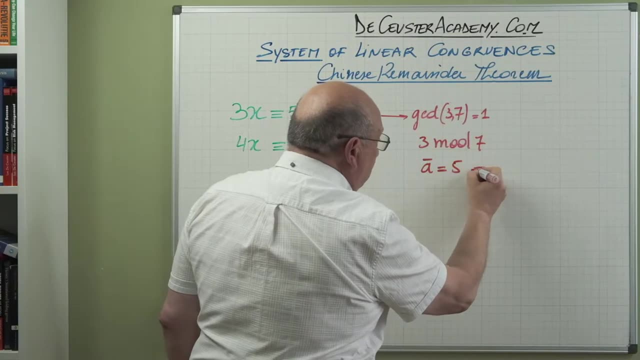 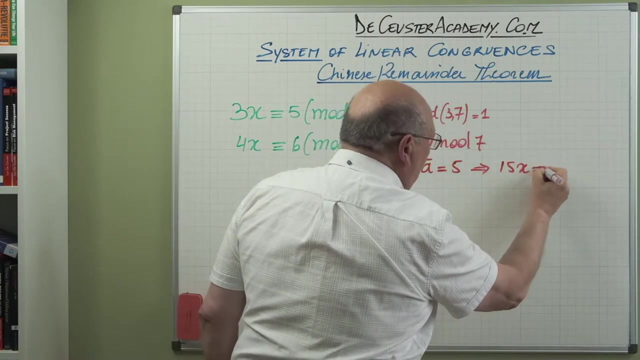 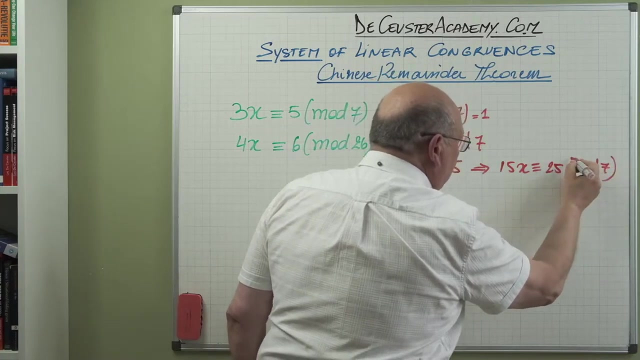 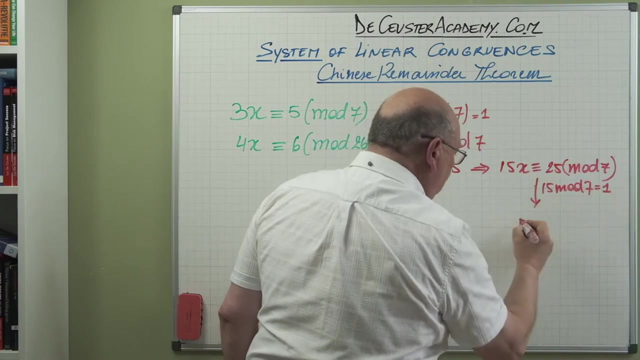 the modular inverse of 3 modulo 7 is equal to 5, so we multiply both sides with 5, we find 15x is congruent with 25 modulo 7, what we know. 15 modulo 7 is equal to 1, so we find: 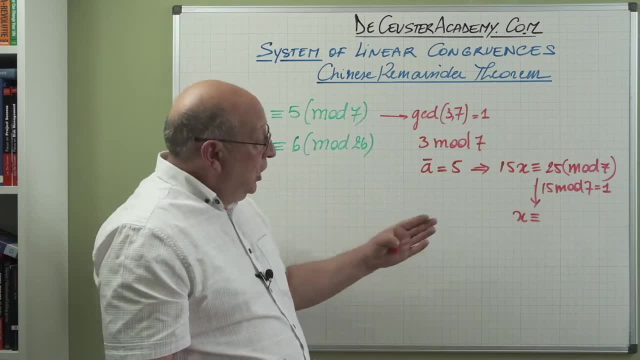 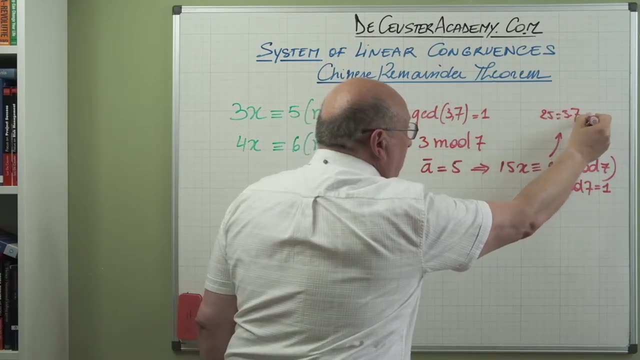 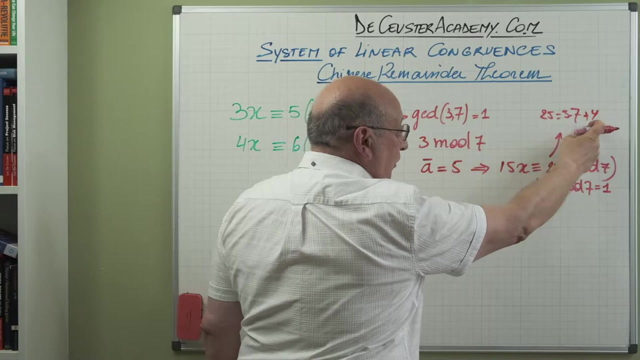 x is congruent 25 modulo 7, but 25 we can also write as 25 is 3 times 7 plus 4, so basically the modulo's 25 modulo 7 is equal to 4, so we find 4 modulo's 7 and 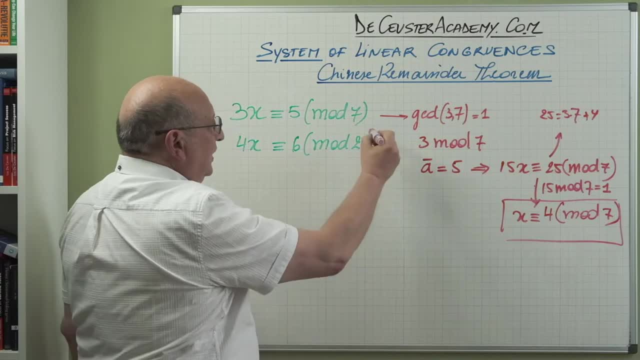 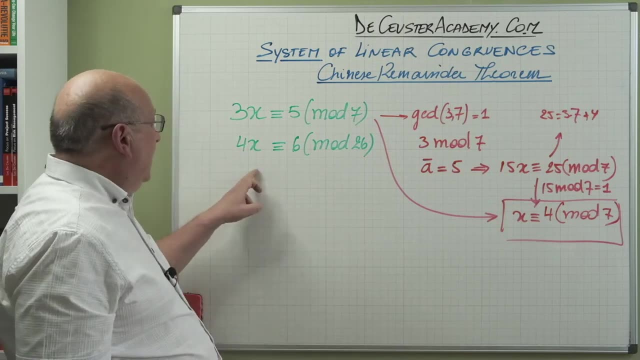 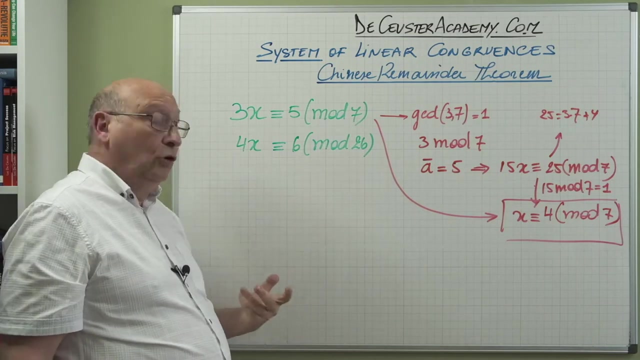 that's basically the first equation that we will use in our system. so that's the first thing that we did. The next thing here: the GCD of 4 and 26 is not equal to 1.. what we have to look at, this we have to see we can say that we have a common 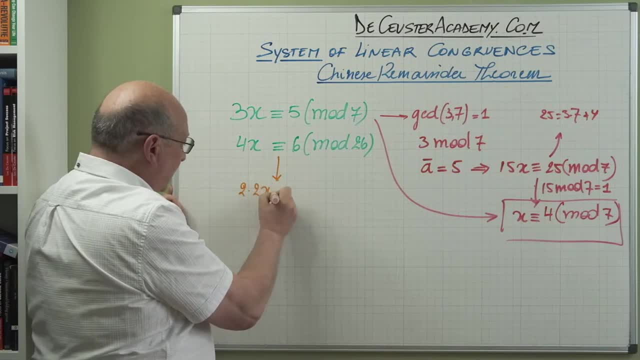 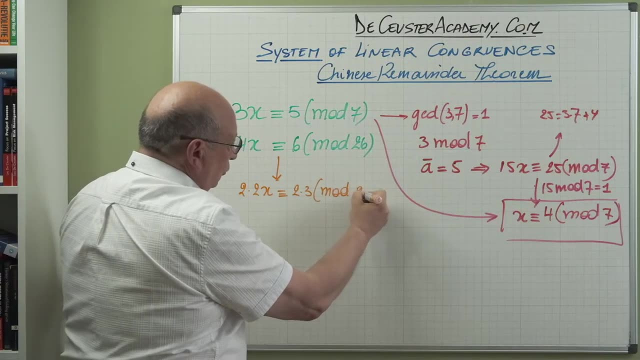 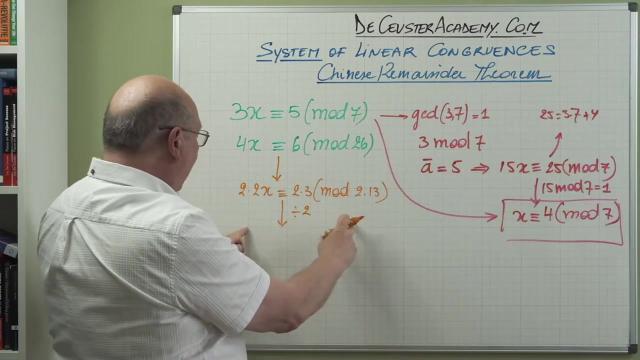 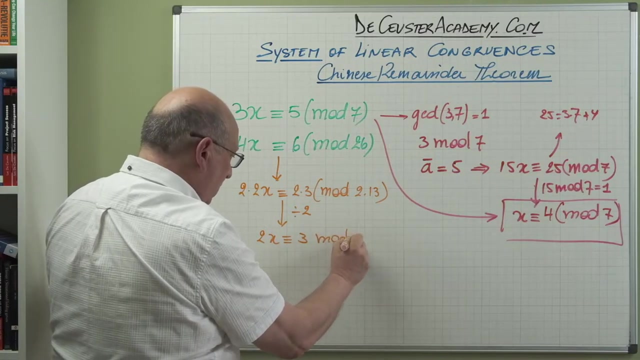 coefficient. so we can say this is 2 times 2. X is congruent 2 times 3 modulus 2 times 13. and what we can do now is divide both members by 2. so I find that 2 X is congruent with 3 modulus 13. and now the same thing. we have to get this. 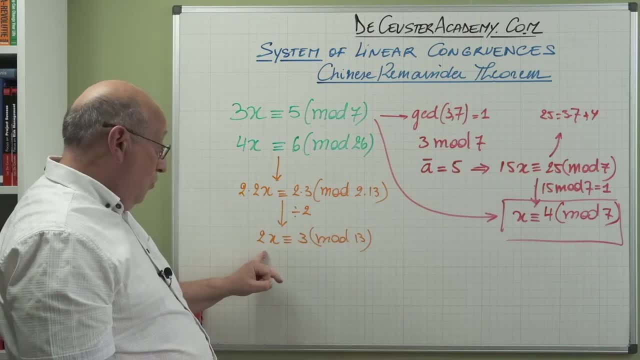 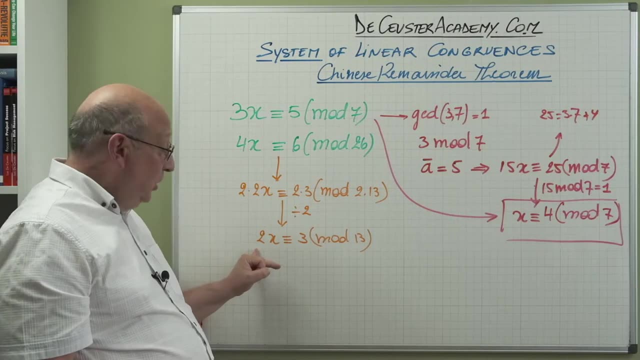 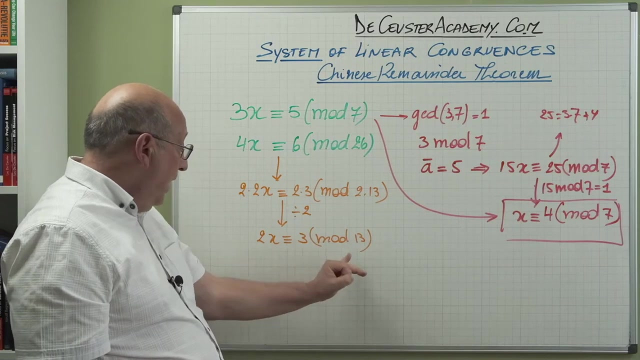 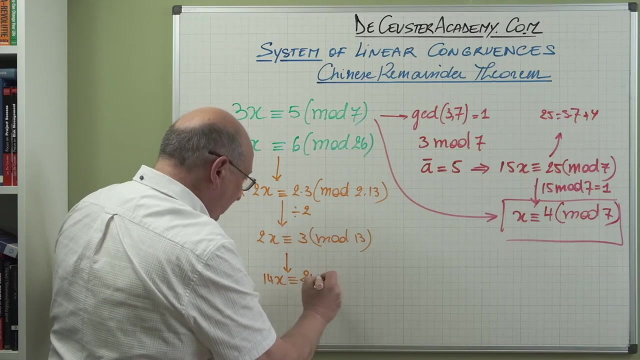 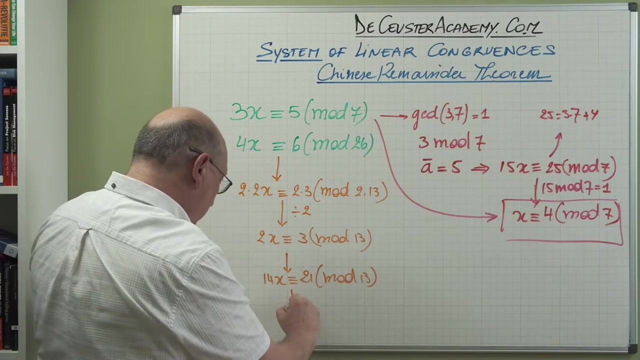 it's still out of this expression. now we see, or we can calculate it. we see: when we multiply 2 with 7, we find 14, and 14 modulus 13 is 1. so when we multiply both sides by 7, 7, I find here 14. X is congruent with 21 modulus 13, and this is equal to 1: 1 or. 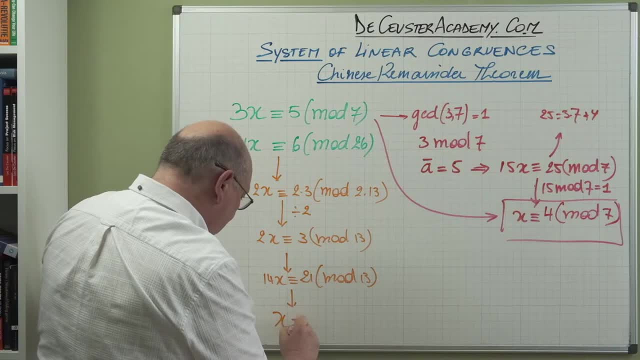 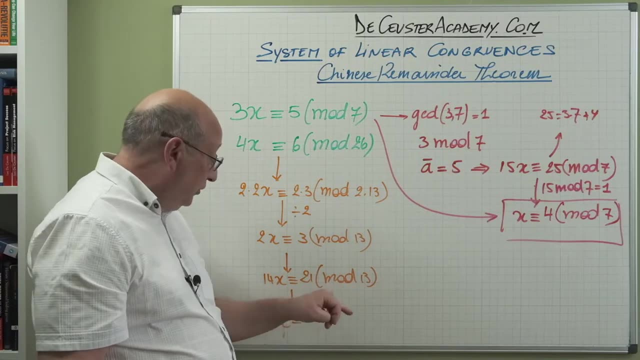 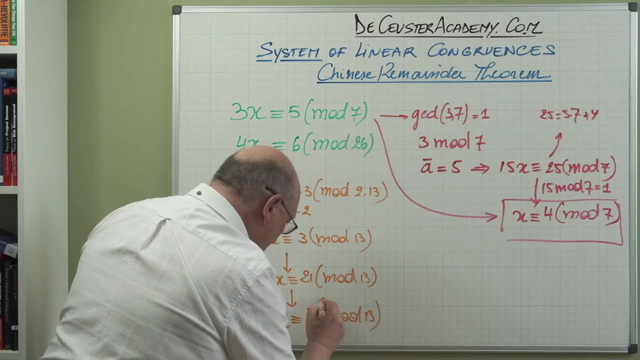 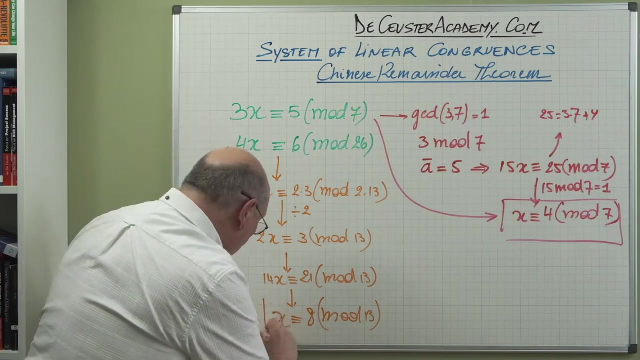 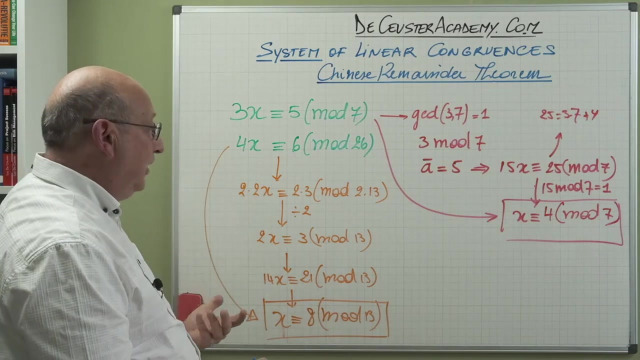 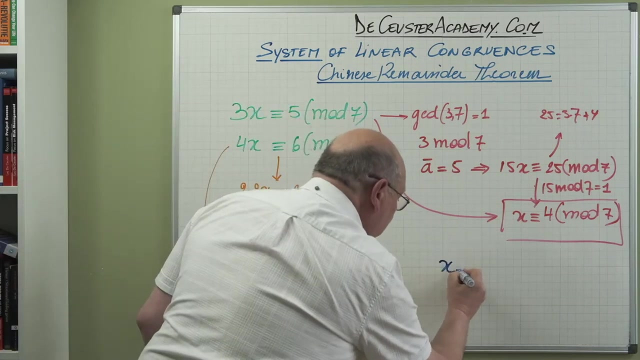 X. we just write X is congruent 21 modulus 13. well, 21 is 1 times 13 plus 8, so the remainder is 8. so we have 8 modulus 8 plus 8. 06, 07, 07, 08, 08. 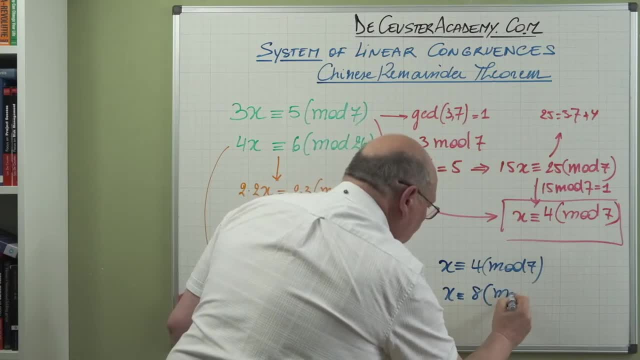 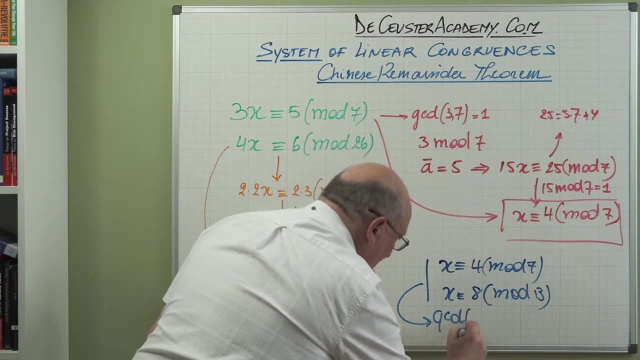 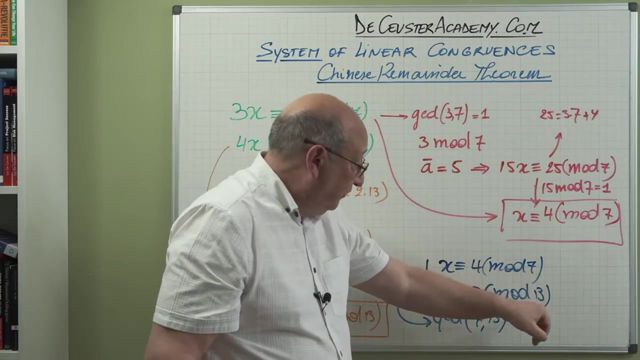 09 010, 013, 018, 019, 020 and 021 021, 36 tienes 016, with 8 modulus 13, and we know that the GCD of 7 and 13 is equal to 1, so I this is logical. 7 and 13 are both prime numbers. of course, they are relatively. 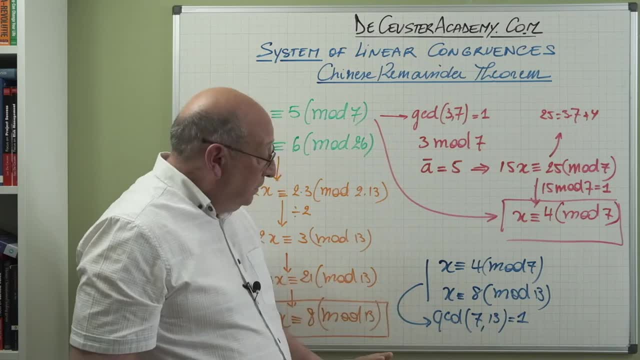 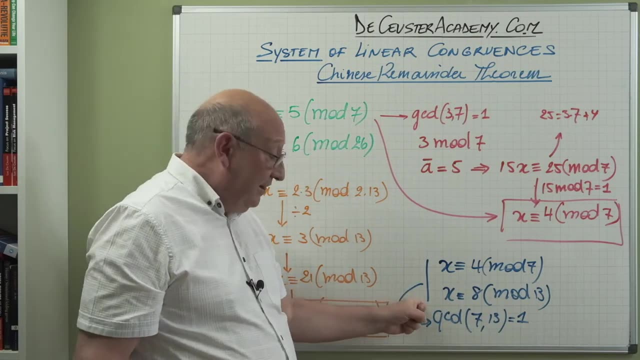 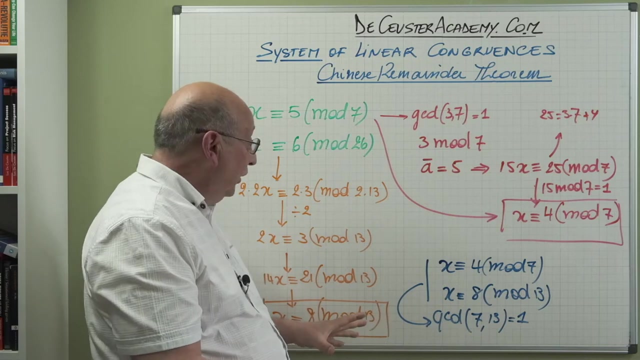 prime. their GCD is equal to 1, and this means that we can find a unique solution for this and this system of linear congruences. and let's do that. but first I have to clear the board so I have more space to do all the calculations we found. 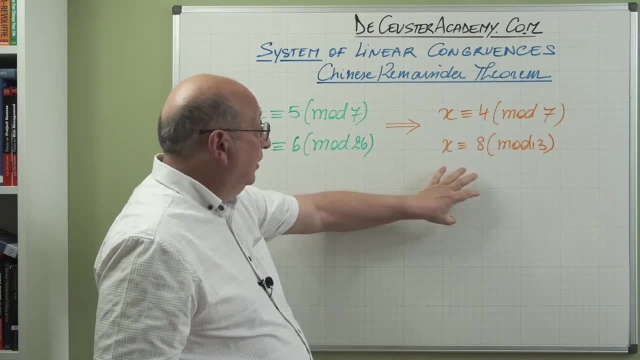 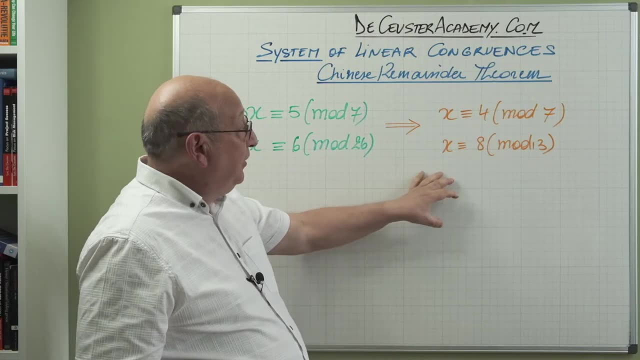 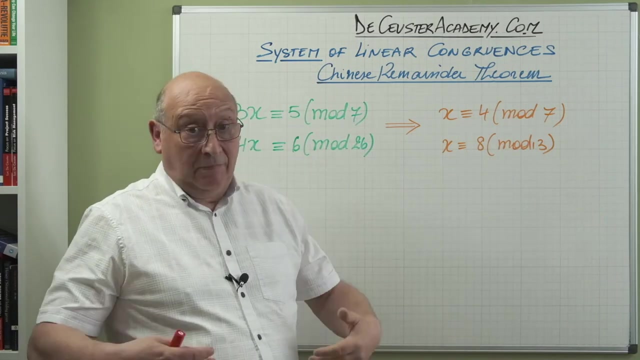 the new set of linear congruences and based on this, we can continue with the next steps. we already verified that the GCD of 7 and 13 is equal to 1 and 13 are both prime numbers. of course they are relatively prime. they're both prime. so that's obvious and we know that. according to the 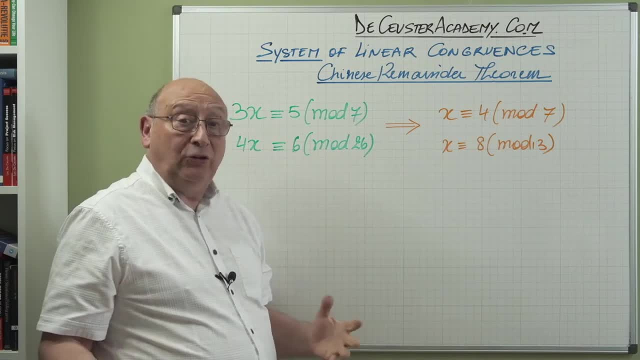 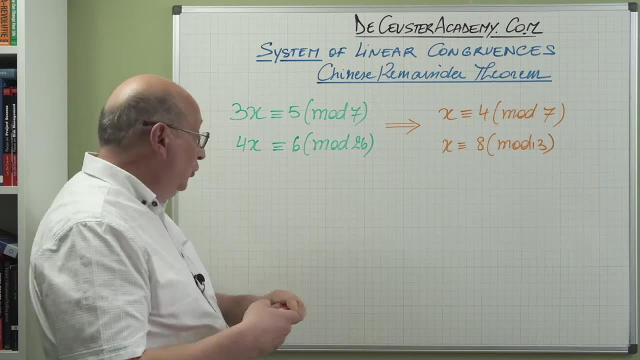 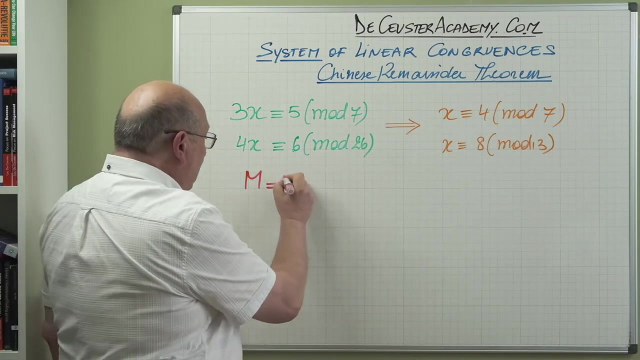 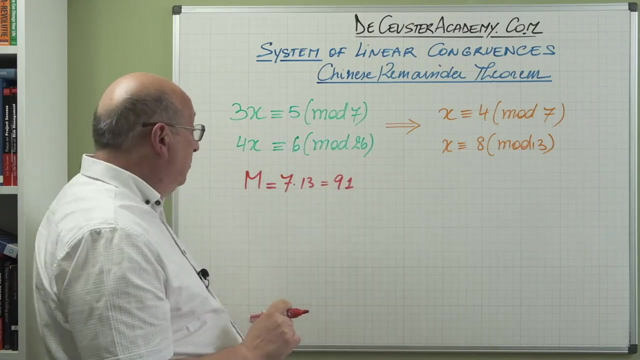 Chinese remainder theorem. we have one unique solution for this set of linear congruences. the next thing to do is to calculate M, the mode, the modular value. so we have 7 times 13, which is 91, so our solution will be congruent: modulus 91. we have M 1, which is 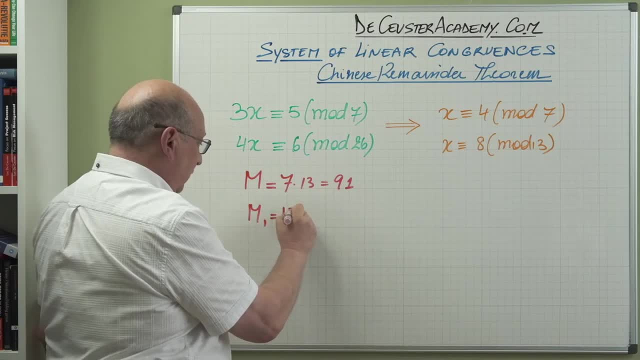 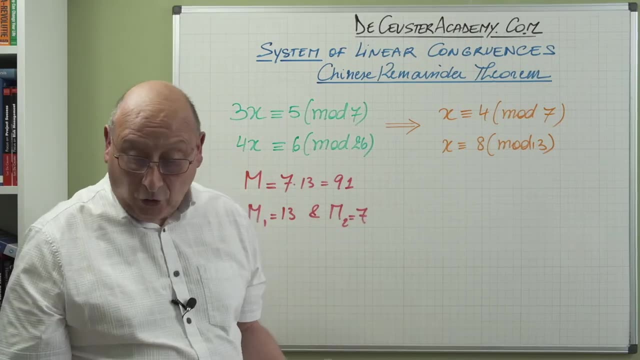 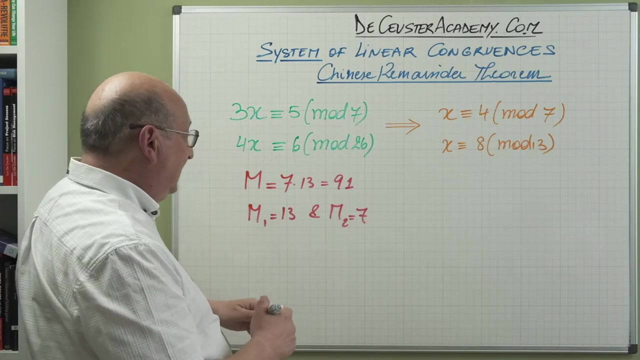 M divided by 7, which is 13, and M 2 is equal to 7. so that's very easy to find, because we only have two numbers here. now, based on this, we can write the new expressions. we can say that we have M 1. 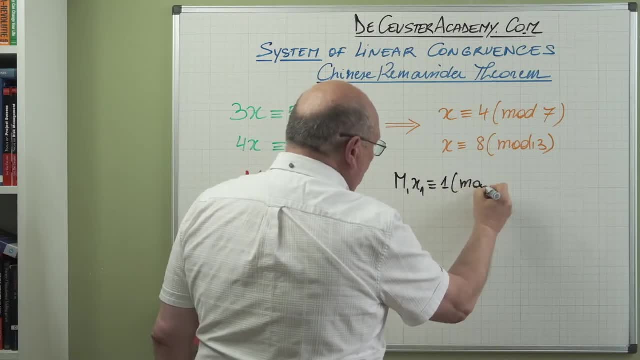 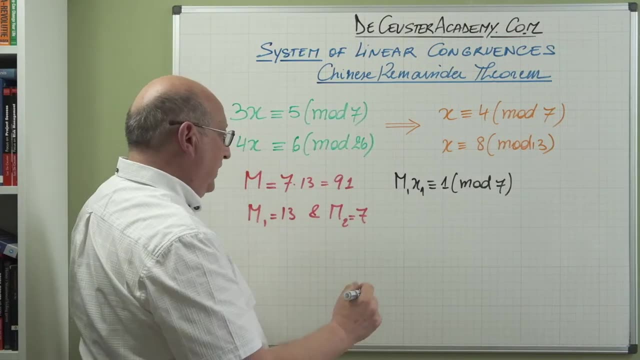 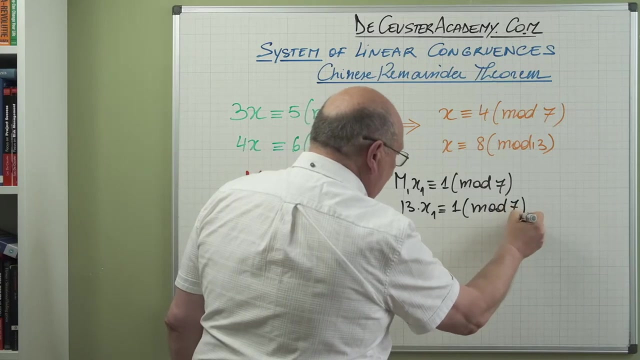 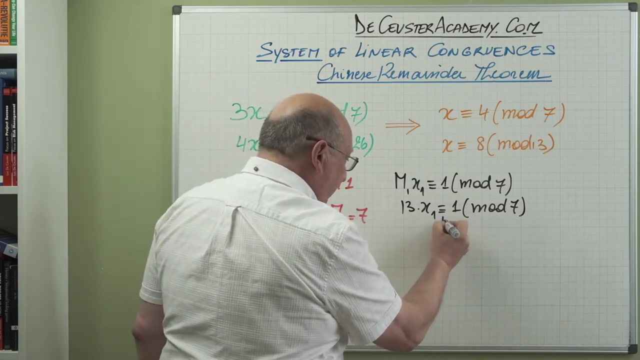 X 1 is congruent with 1 modulus 7, and when we replace the values here, we have 13 times X. 1 congruent with 1 modulus seven. 13 X threatened X 2, make sure, perfectly, очки 7. we can simplify this everything. 모듈루 7, so we have 6x 1. like and remember, E61 is congruent to modul7 7. you can simplify this everything. 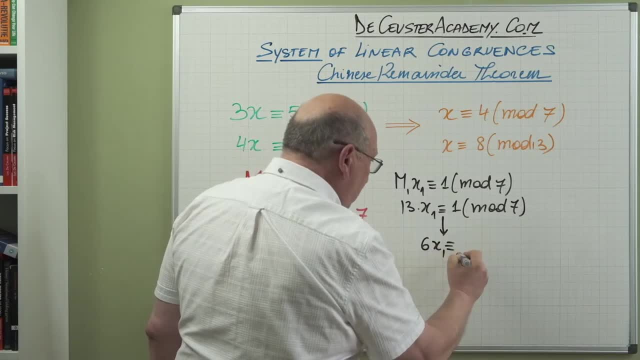 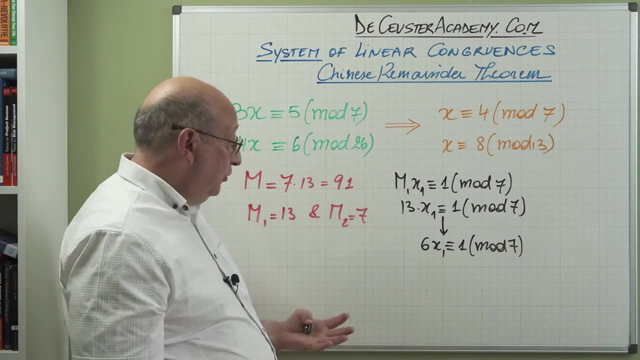 segurança: 7, so we have 6x 1 is congruent to modul7 7. we can simplify this everything: 6AST modulo 7, so we have 6 X 1 is segunda AS. make sure you visible, complex, complex went with one modulus seven and now we have to find the value that gives us. 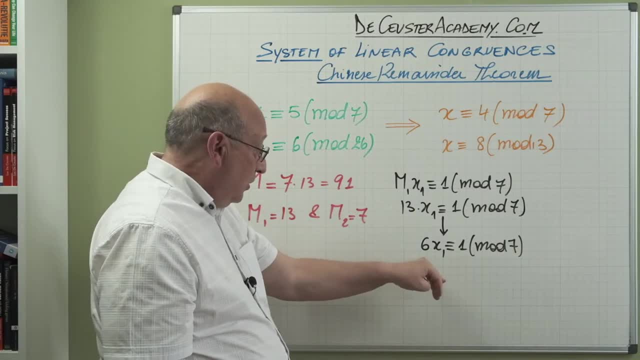 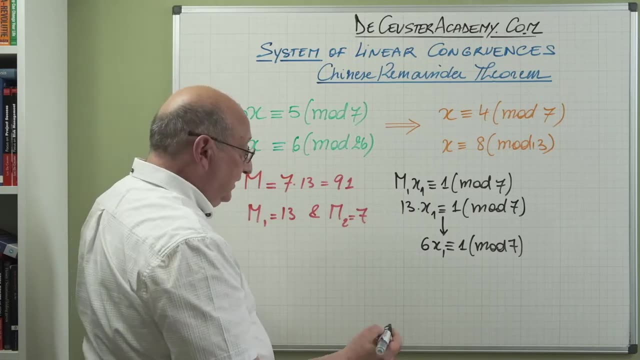 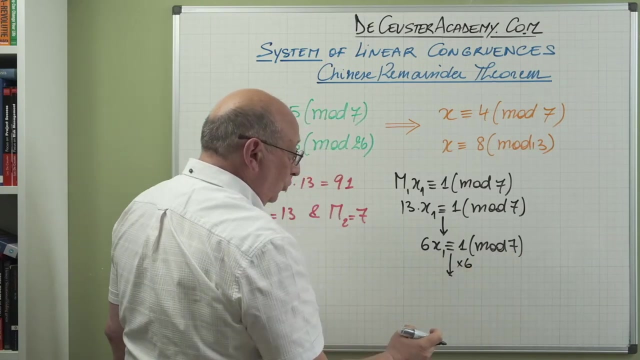 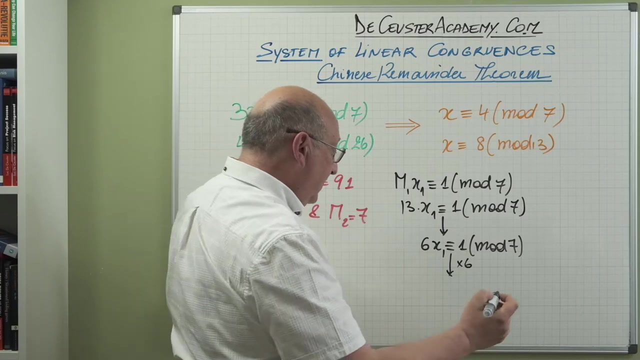 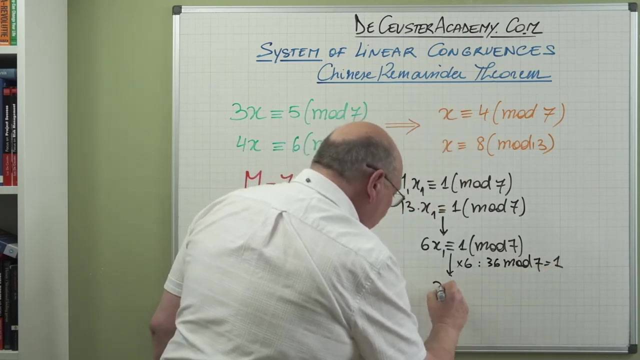 that let's say the inverse, the modular inverse of six modulus seven. so when we do this times 6, 36, 36, when we look at modulus 7, 36 and we have 7, so we have 5 times 7. so basically we can say 36 modulus 7 is equal to 1. so we find X, 1. 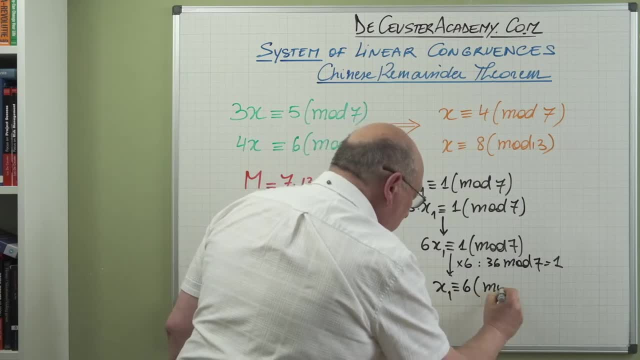 is congruent with 6 modulus 7, and that's 7, and that's the inverse of 6. so we can say: 36 modulus 7 is equal to 1. so we find X: 1 is congruent with 6, modulus 7, and that's. 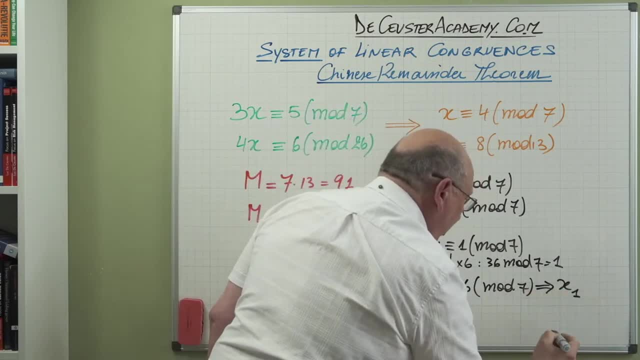 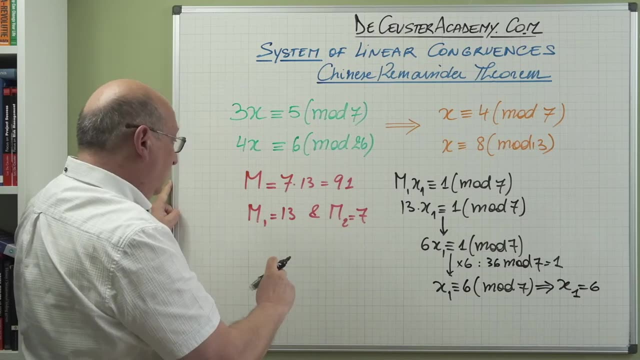 the first value for X 1 is equal to 6. the first value for X 1 is equal to 6. now we do the same thing for m2. X 2 and 2 is 7, so we find 7 X 1, X 2. sorry it. 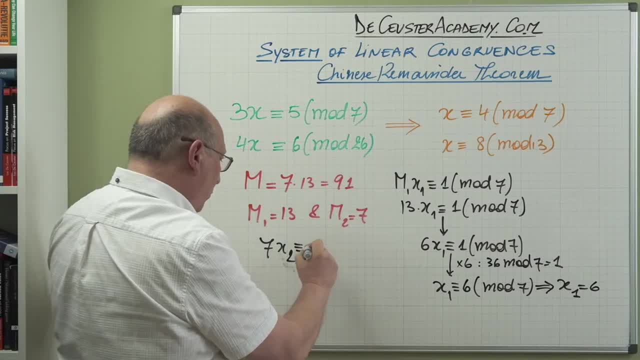 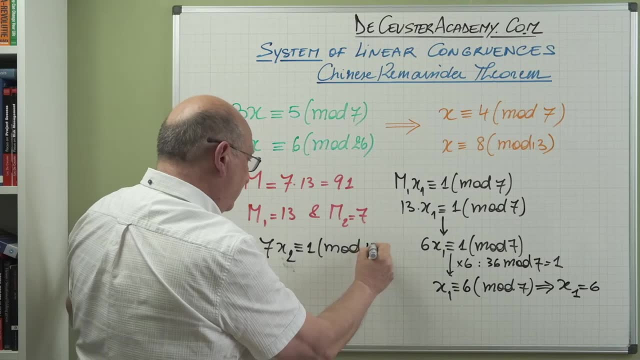 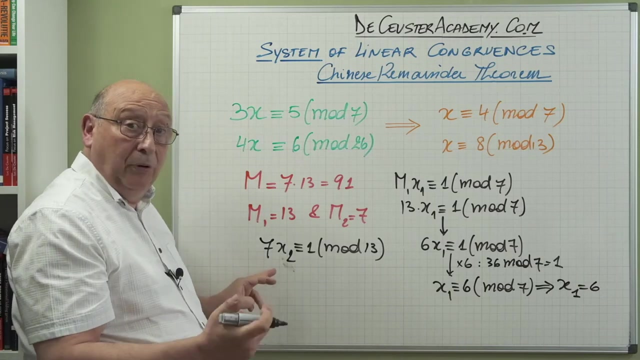 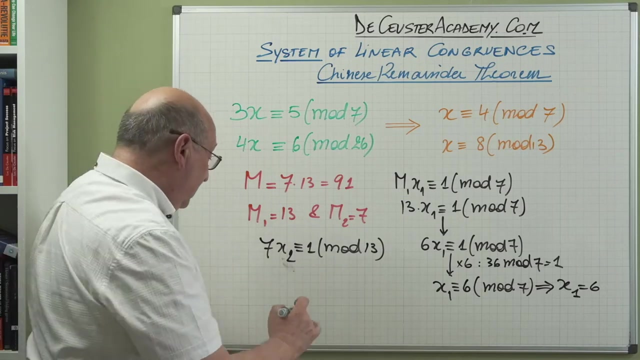 has to be X. 2 is congruent with 1 modulus 13. now and we find here: well, we can see immediately that the inverse of 6 is equal to 6 and that's the inverse of 6. when we multiply both sides by 2, we find we find 14, and 14 modulus 13 is 1. so we 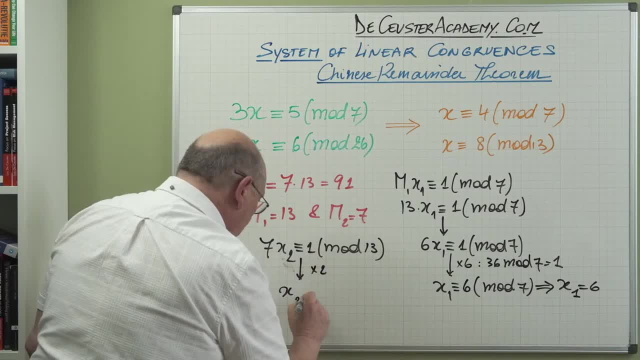 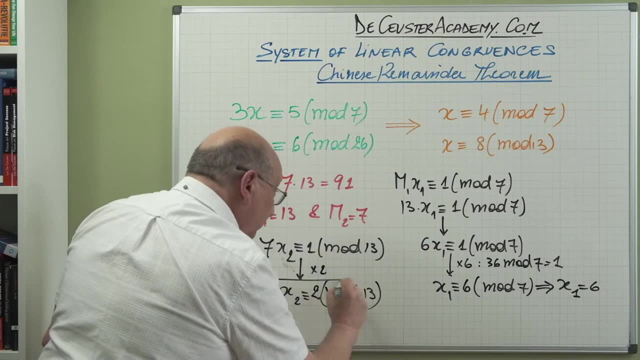 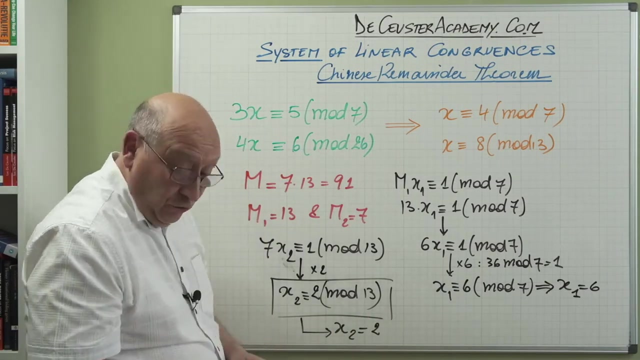 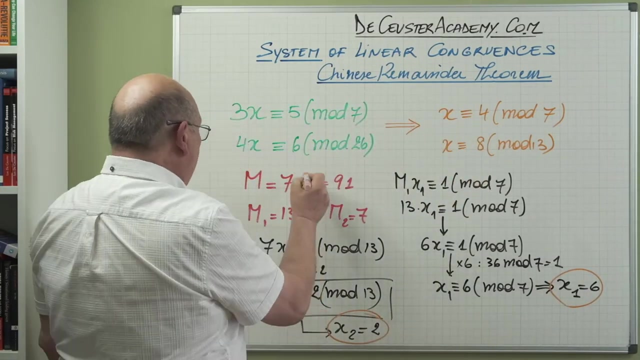 multiply by 2 and we find X 2 is congruent with 2 modulus 13, which gives us that X 2 is equal to 2, and basically those are the two values that we we need. We need x1,, we have x2, we have m, we have m1 and m2, and now we can say: 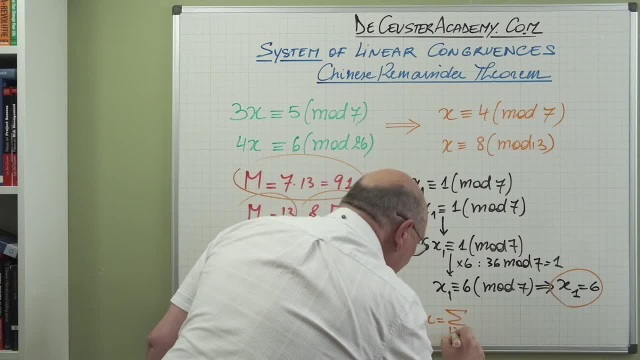 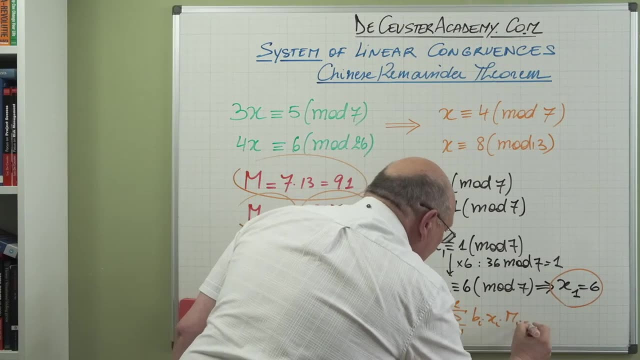 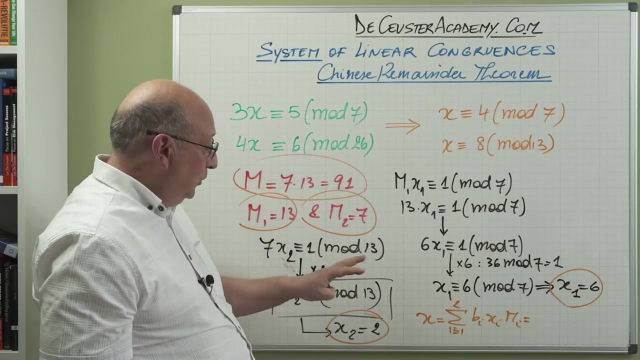 that x is equal to the sum of i, equal to 1 to 2, bi times xi times mi, and we will find the final result here. But before we continue with this, I will make a summary of what we found and then we calculate the final result In the table. 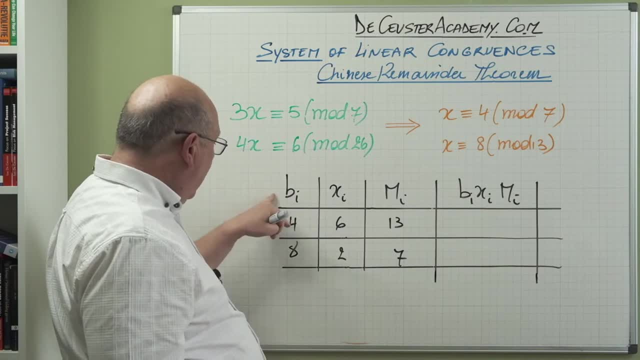 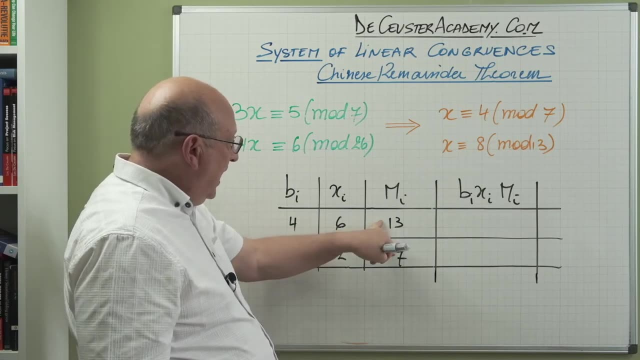 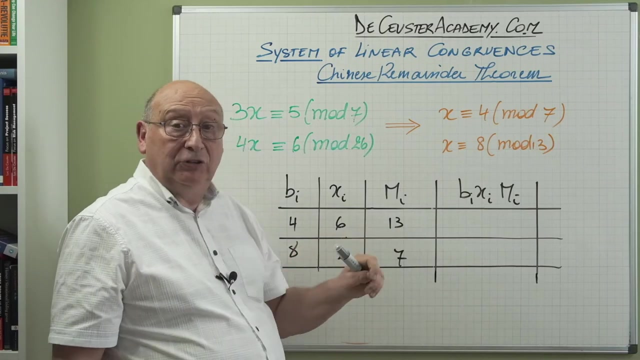 I summarized the results that we had before: bi b1 is 4 and b2 is 8, x1 is 6, x2 is 2, m1 is 13,, m2 is 7.. So when we multiply 4 times 6 times 13,, we find: 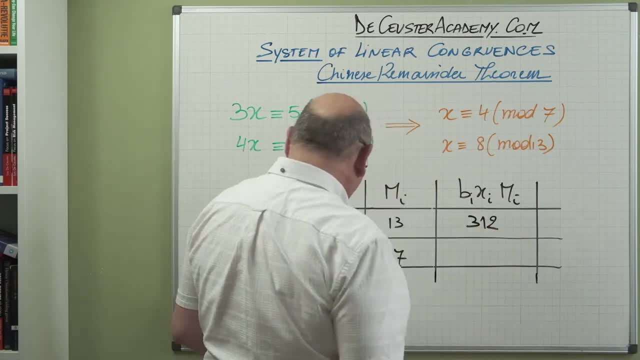 this is equal to 312. and then we have 4 times 6 times 13,. we find this is equal to 312. and then we have 4 times 6 times 13,. we find this is equal to 312. and then we have. 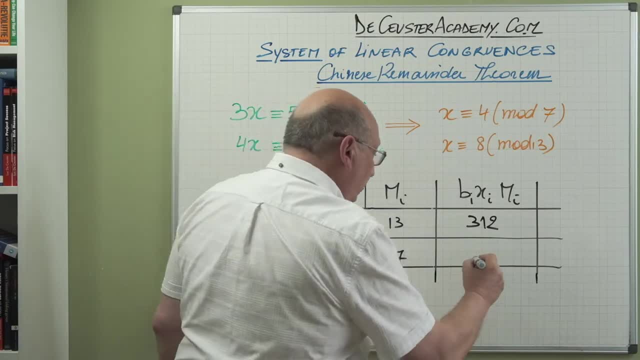 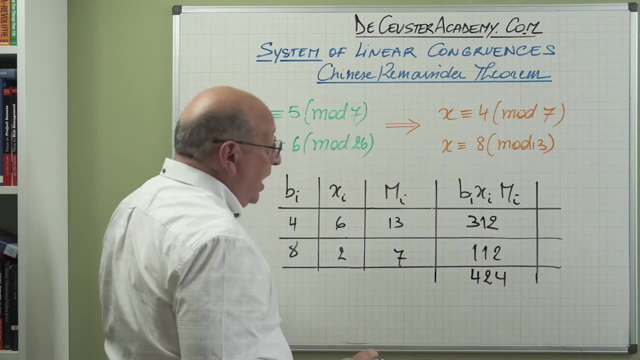 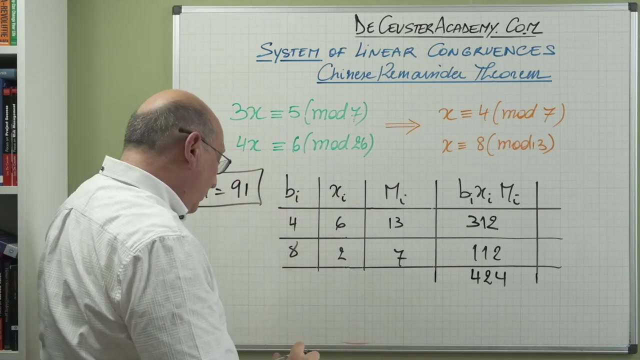 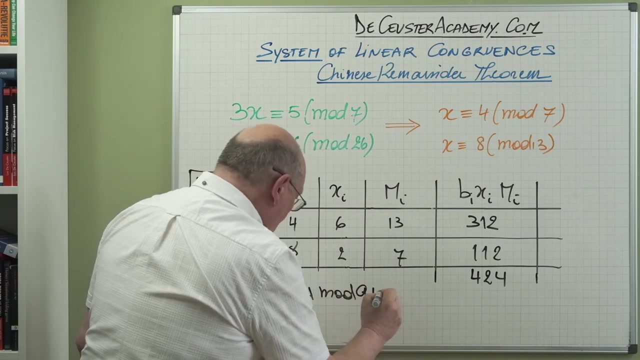 8 times 2 times 7 is 112, which gives us a total of 424.. Now, this is a solution. modulus m and m is 91.. So what we can say? we have 424, modulus 91, which is equal to 60.. 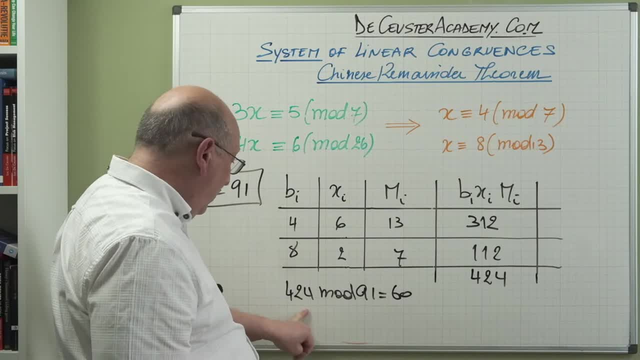 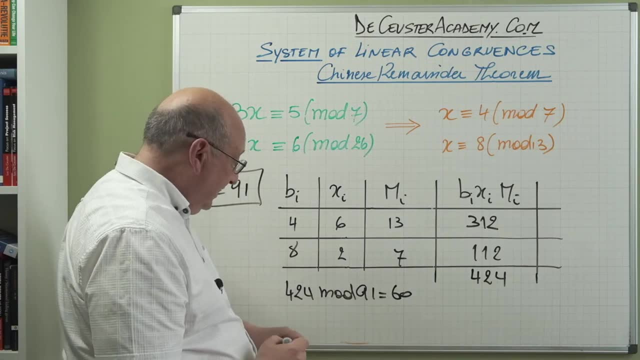 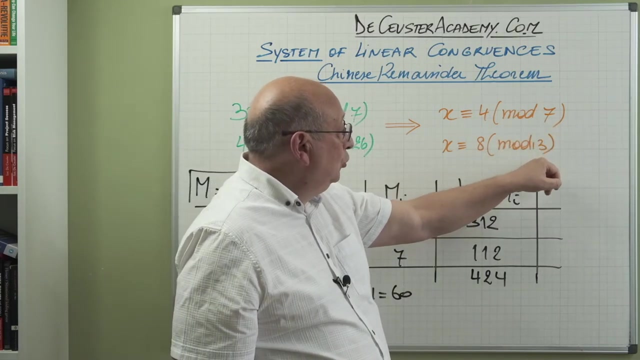 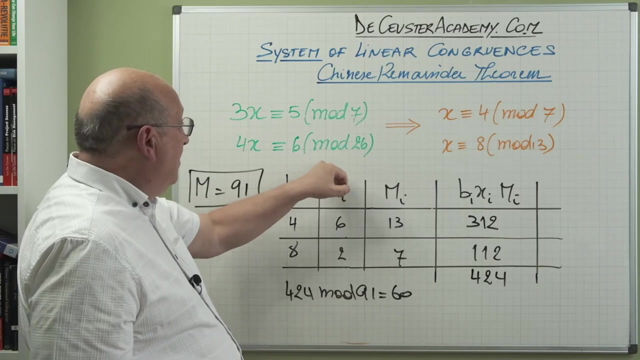 We can say that 424 has a remainder of 60 modulus 91. Now what we have to see here is that we have here 91, which is the product of the moduli of the two reduced equations. But what do we have Basically? originally- m original was the- 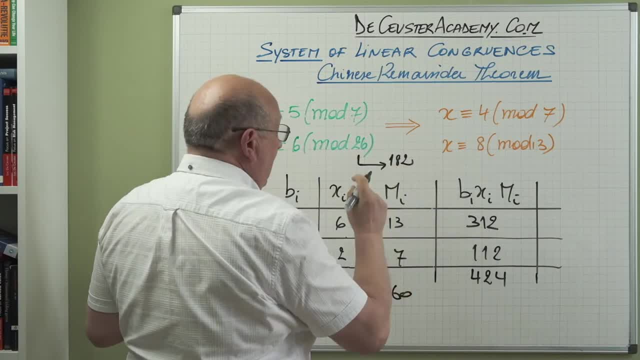 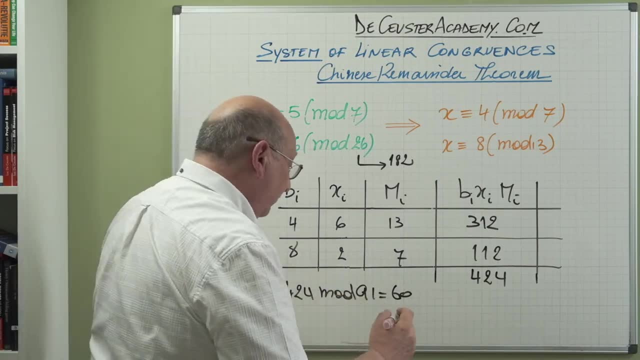 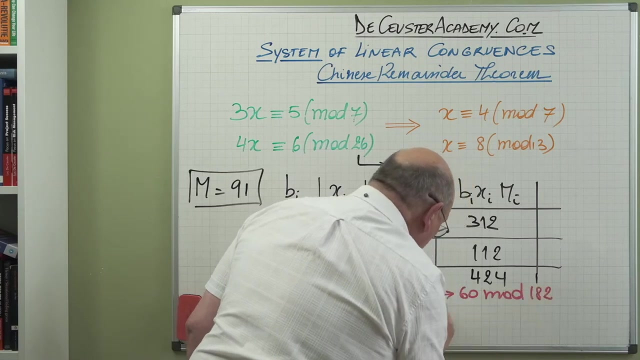 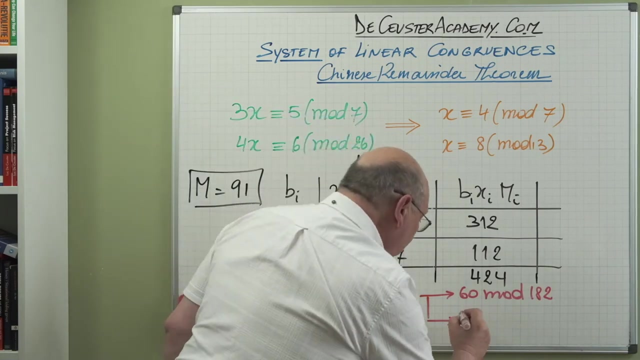 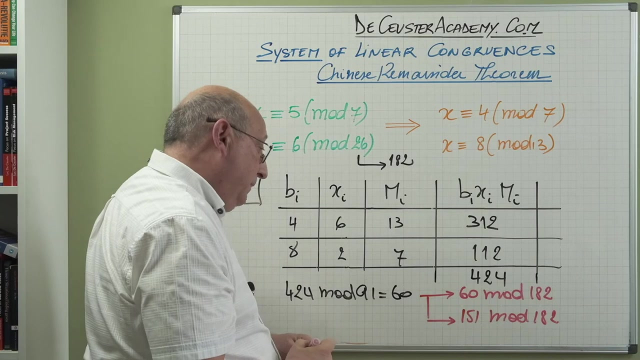 double 182. So basically, we have to adjust the solution to the new modulus, And we have then 60 modulus 182, and the second one- we add 91 to this, because there is a difference of 91, is 151 modulus 182. And but basically we have.